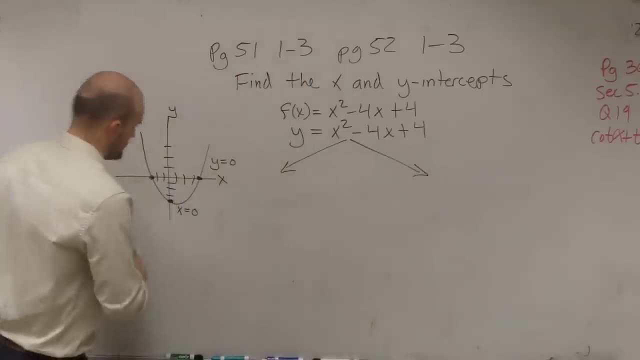 two cases. So the first one, like I said, you don't really this is just kind of a sketch For the first one. I told you you didn't have to draw it. I can help you draw it if you need to. So, when drawing the x and y intercepts, this is what you need to know, Cody: The y intercept is when x equals 0, and the x intercept is when y equals 0.. Now you're definitely going to want to make sure you have that written down. 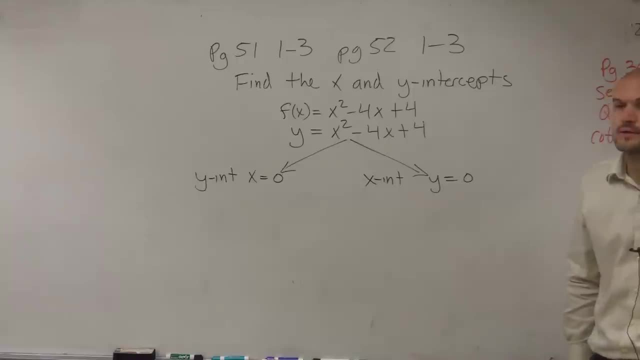 Got it Okay. So all we're simply doing- the only mathematics we really now have to do- is just plug in 0 for either variable. So for over here, when we plug 0 in for x, we have y equals 0 squared minus 4 times 0 plus 4.. And over here we put 0 in for y, we have 0 equals x squared minus 4 times 0 plus 4.. 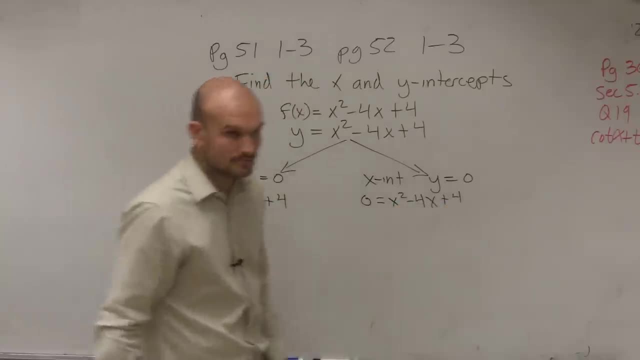 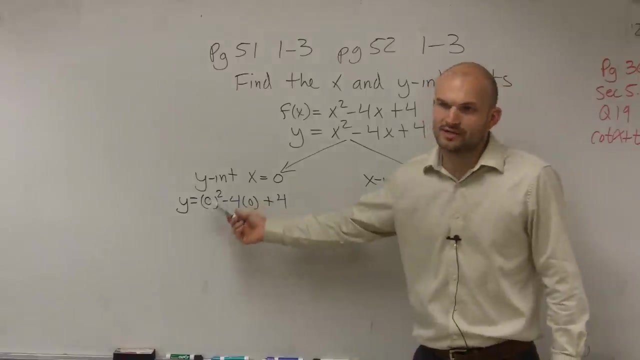 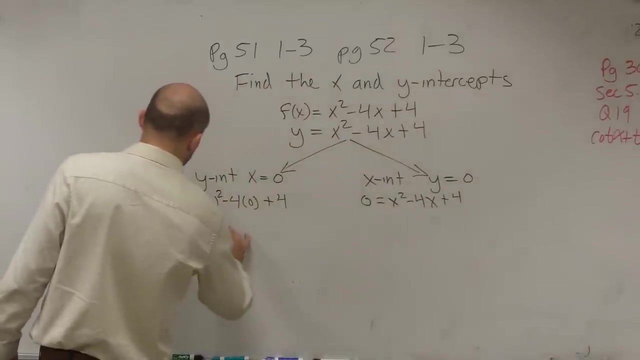 Minus 4x plus 4.. Okay, So now, when looking at this, the y intercept's pretty basic, because 0 squared is 0, negative 4 times 0 is 0, so therefore I have my y intercept is when y equals 4, which sometimes we like to write as a coordinate point of 0 comma 4.. All right, And you guys are going to have to know how to do that and plot it. 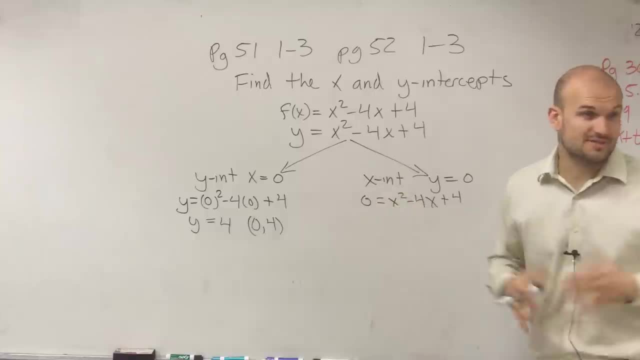 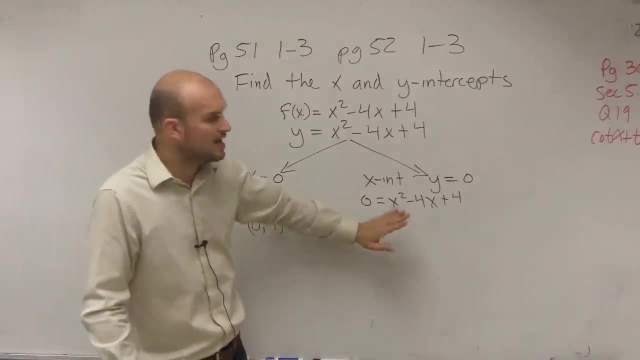 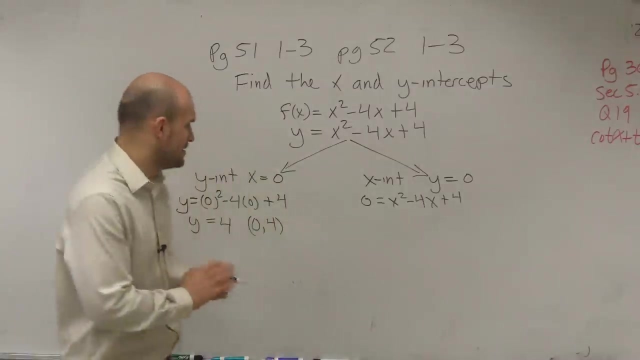 Huh. Now this is where it's going to get a little bit more difficult, though, with the x intercepts, because this goes back to a little bit actually our homework from the previous class. How do we solve for x when we have more than just 1? We can't just get x by itself, but we have to look into factoring. So that is where we're going to go back into this case again right, Where you do your a times c over b. So therefore you look at what two terms multiply to give you 4.. 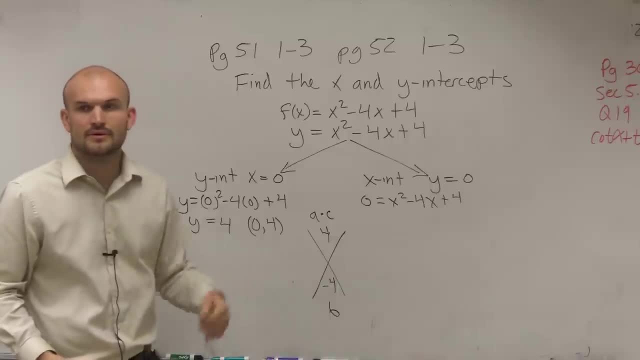 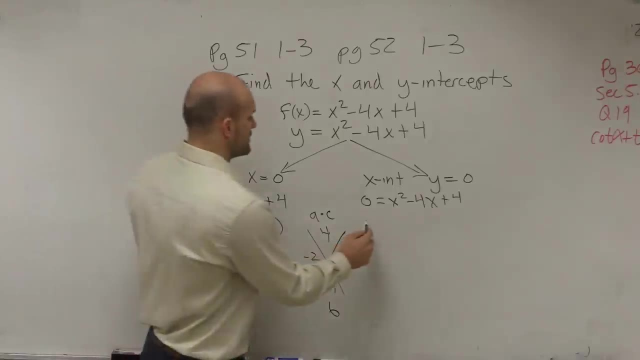 But add to give you negative 4. And you're going to have negative 2 and negative 2.. Therefore, you could say 0 equals x minus 2 times x minus 2.. By applying the 0 product property, we can say x minus 2 equals 0 and x minus 2 equals 0. Therefore x equals 2..